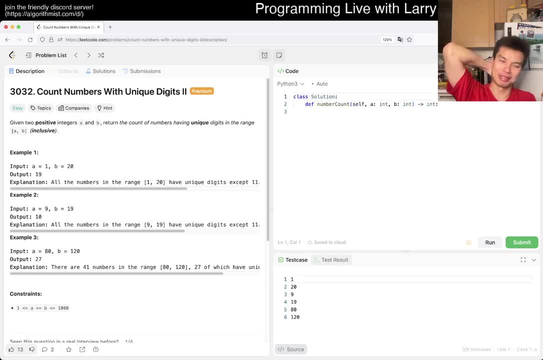 And the layout always annoys me. Sorry. A Yeezy one, Dirty dirty. Two Count numbers of unique digits. Two, A Yeezy bomb And, of course, the explanation I have to kind of I don't know. What is this. I feel like it used to like I don't know. Am I wrong? This layout is so bad. I mean, I feel like they test this but ignore people. who goes back because it's so bad, Like is there a? I don't know? 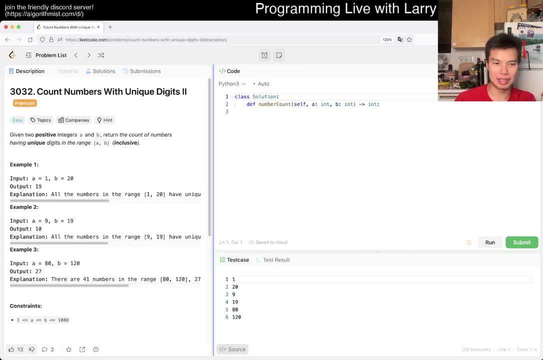 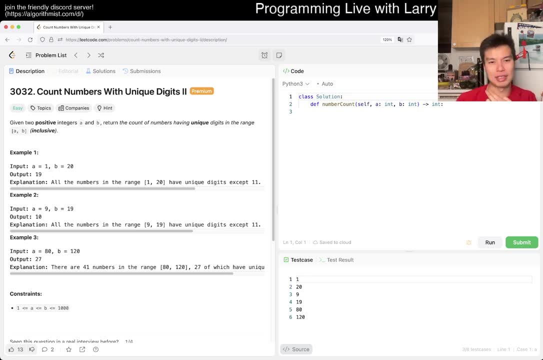 Just like I can't even see my department. one thing Anyway. All right, Let's actually read the bar. Given a two positive integers, A and B, we turn the count of numbers having unique digits in the range A and B, All right, So basically we're just trying to remove duplicate digits, Or like numbers with duplicate digits. I mean, it's kind of interesting And it could be an interesting problem, But the thing is that you know the 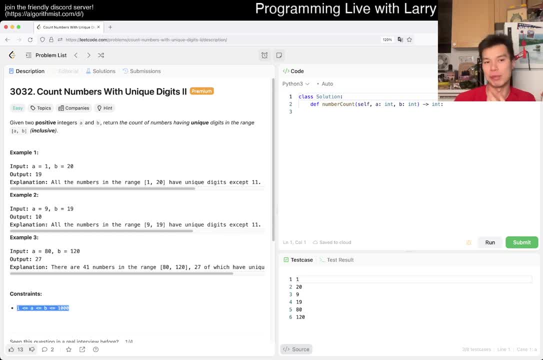 constraints up to a thousand, which makes it easy, because then now you can prove force, because each number has at most three digit, except for 1000, where it's four digits. So because of that, you know, it's just way fast, But I'm trying to think what would be. 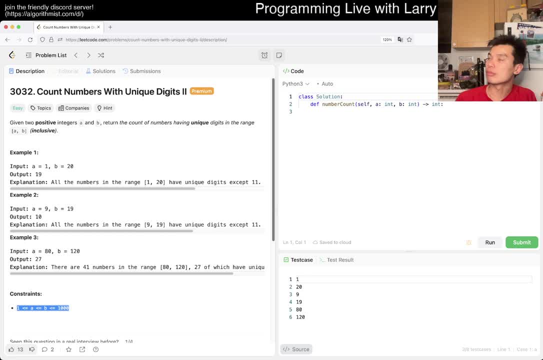 I think the way that I would think about this one is a digit DP. if it wasn't easy I could have more digits and I'm relatively sure because they're really maybe you don't even have to. I mean nine factorial or, like you know, 10 factorial. at most, Nine factorial is 36 or 362,000. That's even if you don't do DP. that's good enough. But if you do DP then you know this could be a bit mask DP and you could do like that kind of counting and making sure that is like a digit DP with bit masks, which is kind of annoying. 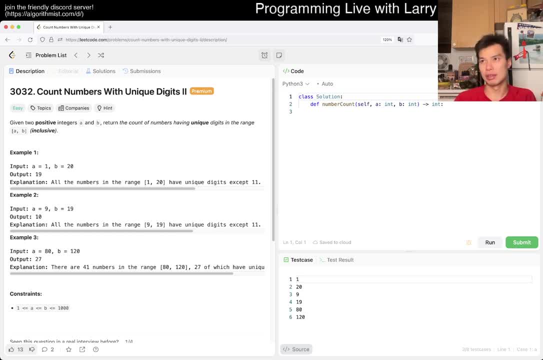 But not impossible, I suppose. Yeah, I mean it's just annoying, I think it's just practice. But for this one we can just do a straightforward count: zero, zero for x in range from a to b plus one, And then, if good of x, right, and then we just return count, And then now we just define good as the function that we're given, which is: 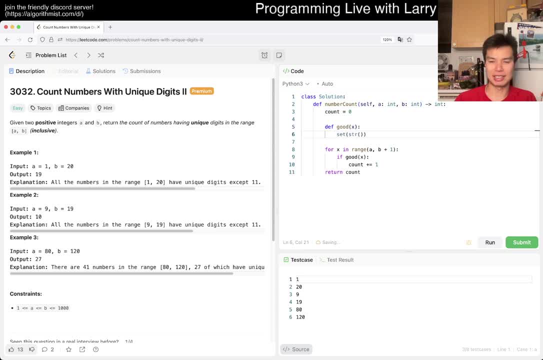 maybe I don't know, I don't know if I can write it quite like this. right, We'll give a spin And after oops, We're basically just saying that you know? Yeah, I mean it looks good here. I'm going to submit it again. I don't know why. 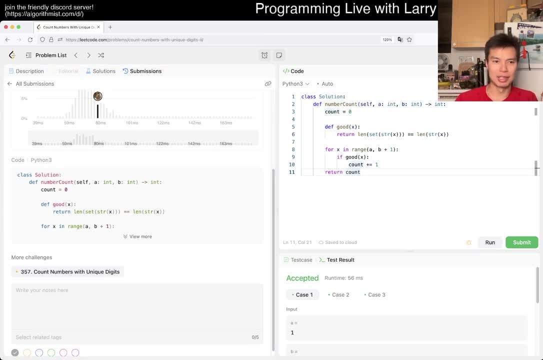 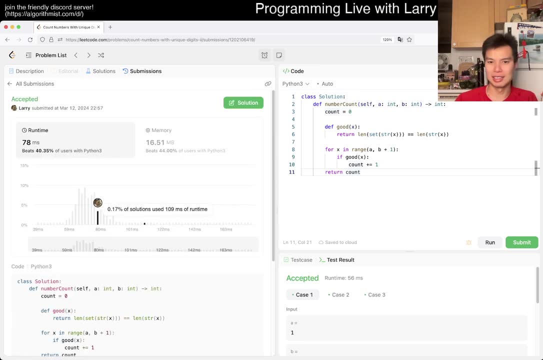 At least it's syntax highlighting seems good this time, But again, I don't know why I need to see the same code twice. Okay, look, there's my face. I don't care about this, Just like I got to go back to the. I don't know, It's just so weird. 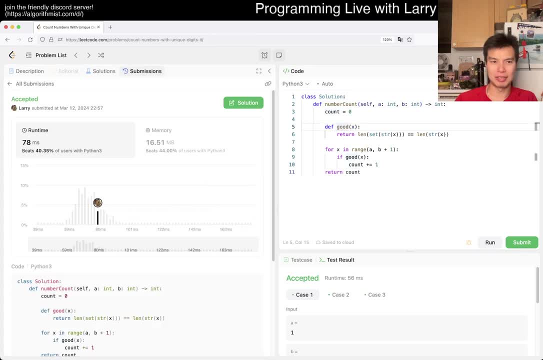 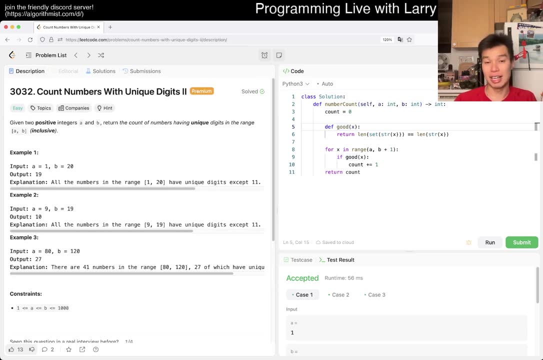 Like: why do I need my if I submit? and what happens if this is a wrong answer? I don't know. Like, why does who is asking for this? Anyway, that's all I have for today. This is going to be. 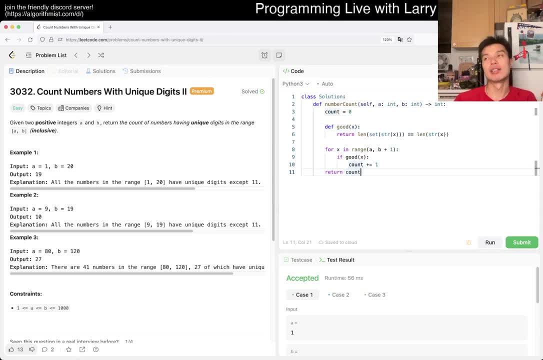 exponential time because, remember, the size of the input is the number or the number of bits representing the input. And in this case we, you know, yeah, we do a lot of digits, So it's going to be exponential. 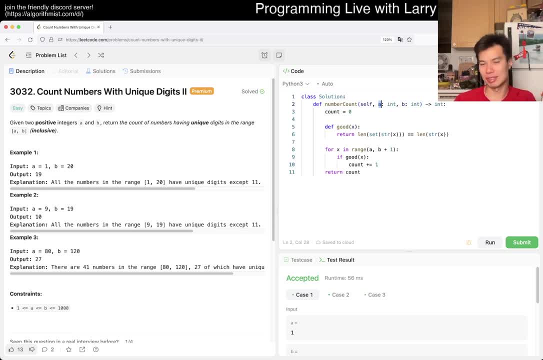 Something like I don't know, log base 10, or 10 to the n or something I don't know. But you only have like: oh yeah, looks like base two like, but I'm too lazy to figure it out, But it's exponential. 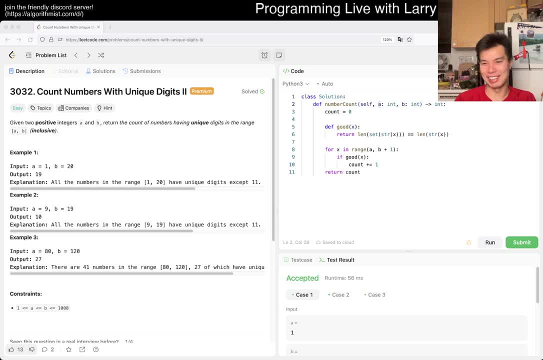 Sorry, friends, I don't know. this layout is just like really annoying me. So my apologies, But that's all I have for this one. Let me know what you think. Let me know if you know someone that can get me a refund on my premium, because this layout is just like I don't know. I don't know how to get it. get back to old one. If you do also know that, let me know. But but that's all I have for this one. 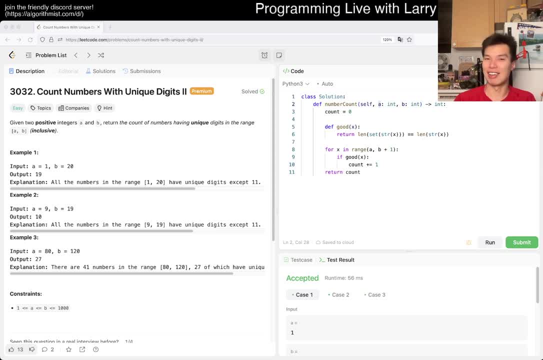 Let me know what you think. Stay good, Stay healthy to go. mental health. I'll see y'all later. Take care, Bye, bye.